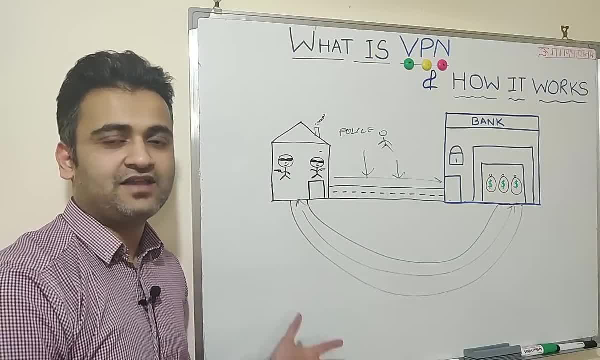 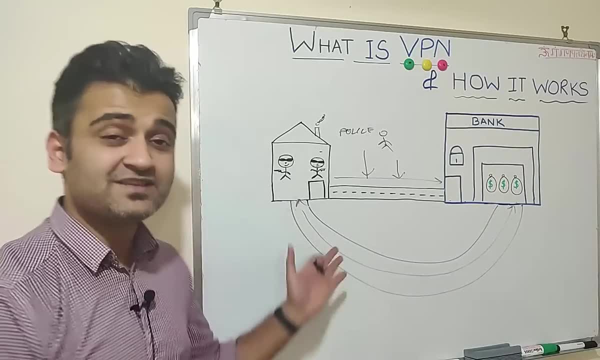 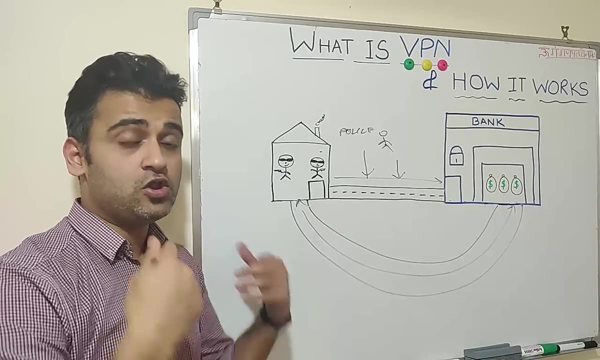 and then come back robbing the bank. this is a famous technique which many robbers have used in various movies, including one of the famous series money heist in Netflix. so, in a similar way- not in a negative, but in a positive way- VPN exactly does the same thing. it it helps you log into a public network anonymously. 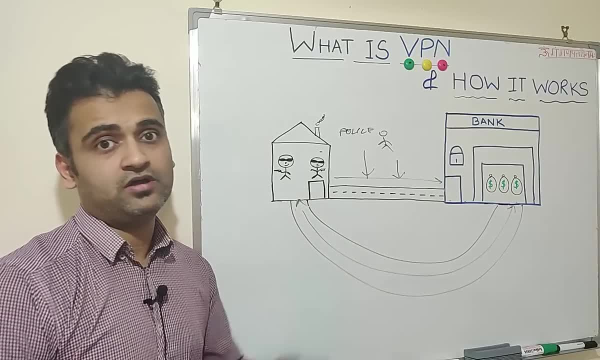 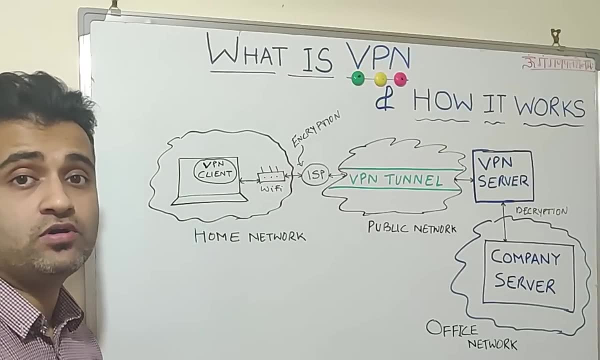 and privately, without anyone coming to know about your credentials and about your location. so let's understand how. so, in order to work from home, you install a VPN client on your laptop, and this VPN client establishes a VPN tunnel, a virtual private network within the public network, which then connects to. 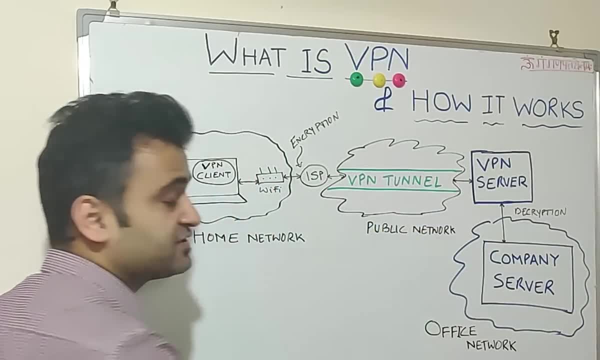 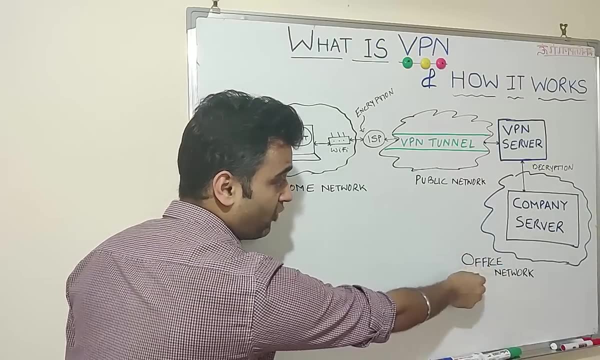 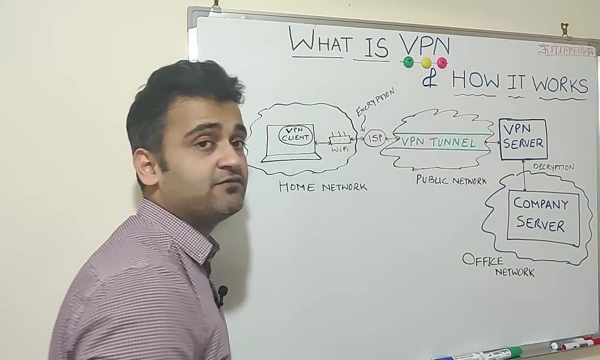 the VPN server and then from the VPN server it connects to the company server. so you send your information from your home network via public network to the office network. but the difference between a normal connection and a VPN connection is that even while traveling within the public network, 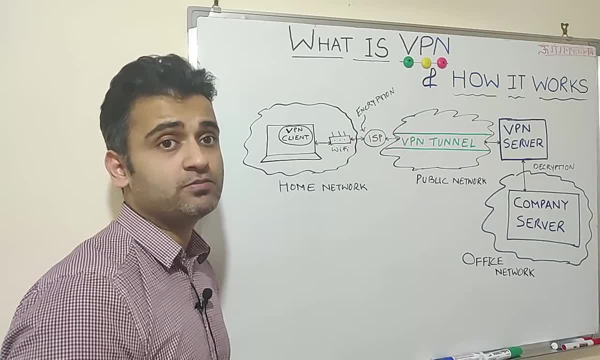 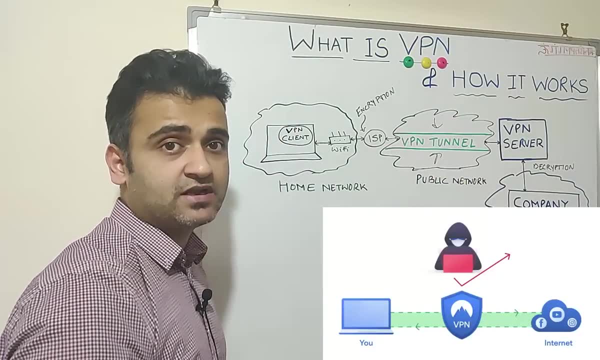 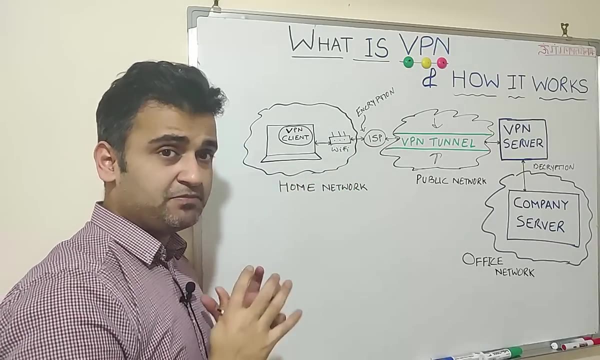 your data and your information remains completely anonymous, completely unknown, so that there could not be any attack from the outside network within this VPN tunnel. so in this way, a VPN network enables all your information to be completely secure from the outside world and basically what it's you know. 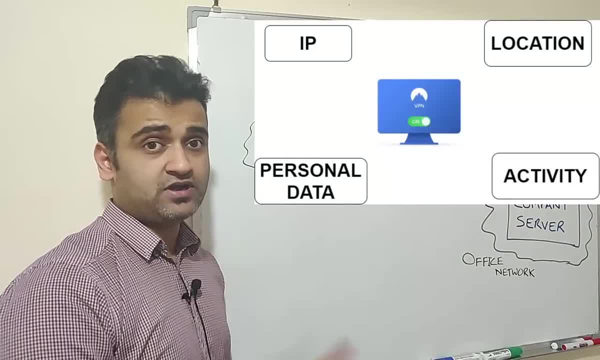 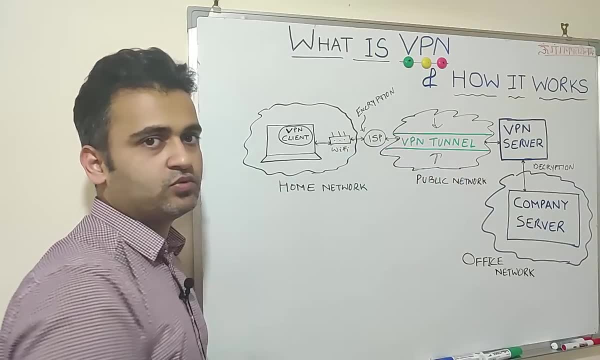 IP address. its ruler key, secures all your important data, what you are trying to send to your office network and vice. at no point of time the outside uh network or people sitting in the public network could know that from where the request is coming from and where it is going. 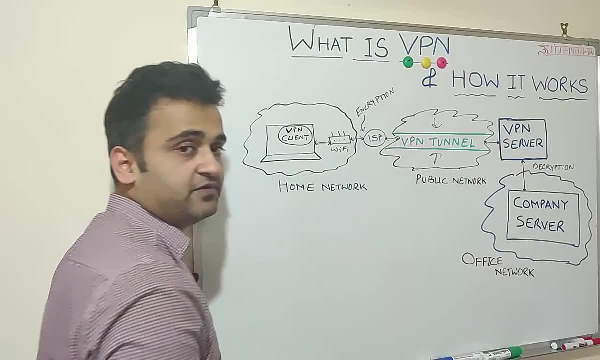 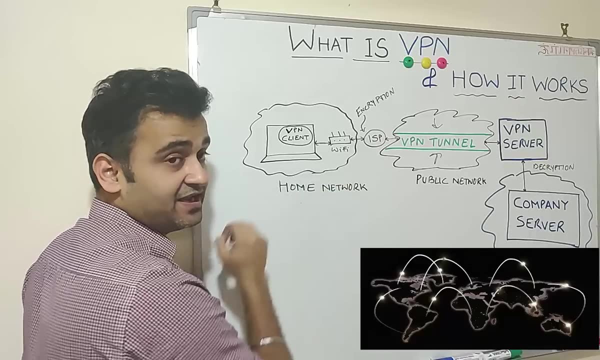 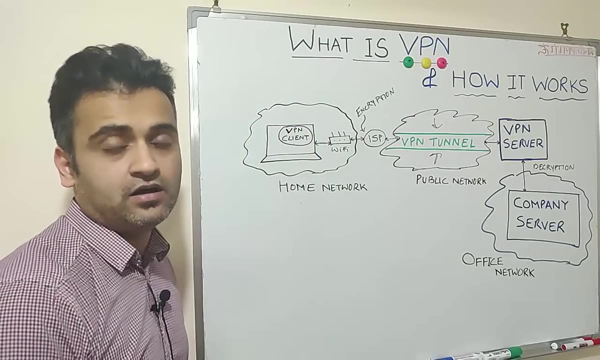 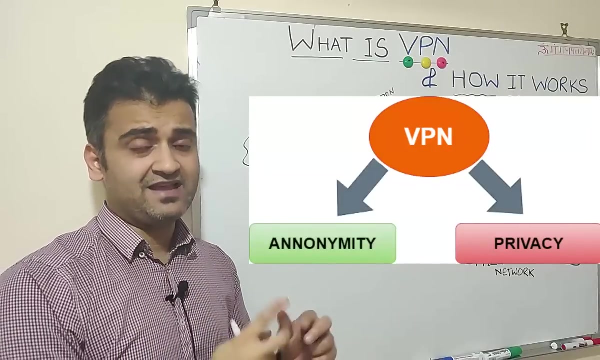 because it is completely managed by this particular vpn server and it can very well be possible that you might be accessing your office uh network sitting in india, your vpn server might be somewhere in europe and your actual office is somewhere in united states. so basically, two things uh vpn provides, which are the two main benefits. first is anonymity and second is privacy. 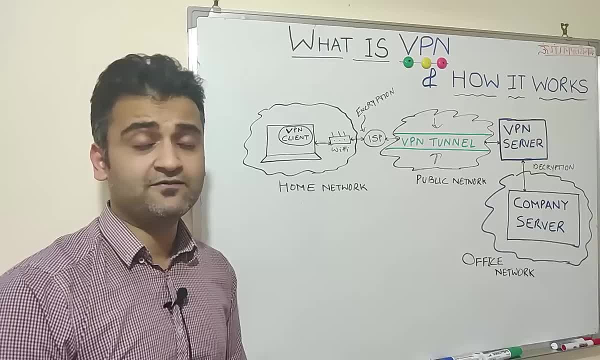 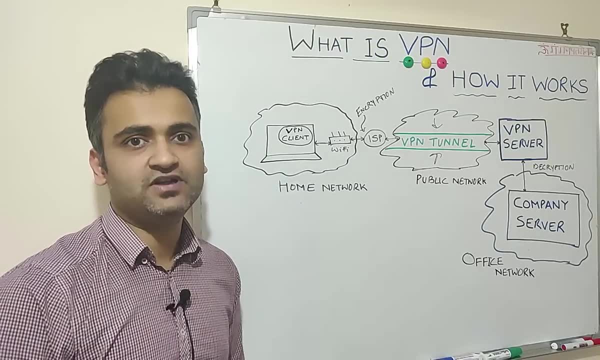 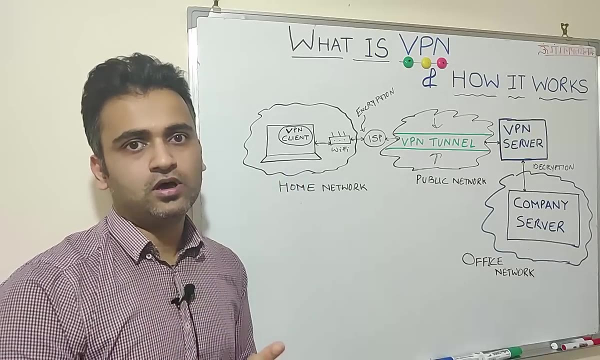 anonymity means hiding your identity: from which location you are accessing what, what is your ip address and all those information and privacy is hiding your activity: which websites you are visiting, what kind of work you are doing on your personal machine. these two uh benefits vpn provides. now this is a scenario for uh connecting to your office.